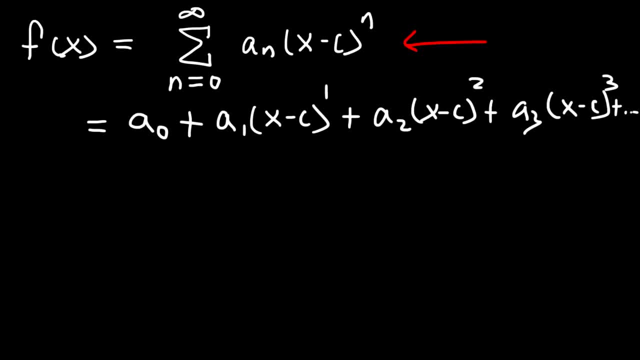 Now, because this is a series this will go on forever. Now, how can we differentiate a power series? So, for instance, what is f prime of x? Well, this is going to be the power series going from one to infinity, and we just got to find the derivative of this. 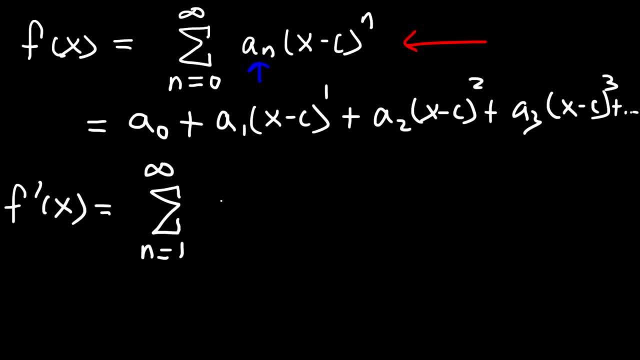 a sub. n is a constant, so we could just rewrite that. Now we need to use the power rule on x minus c to the n, So we got to bring down the nth power, so we're going to multiply the constant by that And then it's going to be x minus c and then we need to subtract the exponent by one. 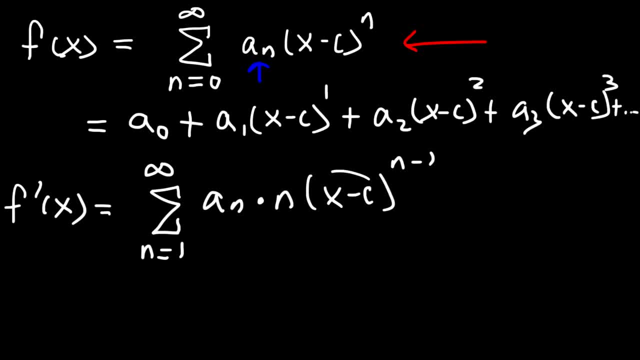 So raised to the n minus one times the derivative of the inside, which is just one. So we don't need to write that Now. to write out the series or the terms in a series, we could do one of two things. We can plug in the n values or we can just differentiate. 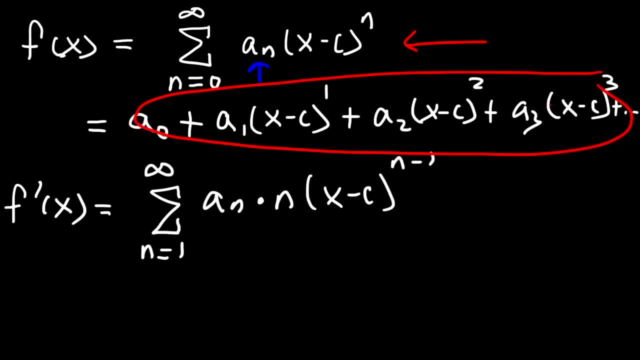 We can find a derivative of a to the n. We're going to subtract distance from the original power series, from a to the n, The derivative of a sub zero, which is the né coastient, which equals 0, and the derivative of this term. you have to ask yourself what is the derivative of x minus c to the first power. 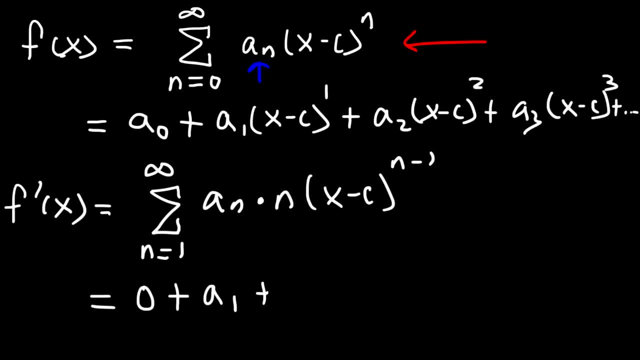 So the derivative of x minus c is one times the constant a sub one. The derivative of x minus c is one times the constant a sub one. Now the derivative of x minus c squared is going to be 2 times x minus c to the first power. 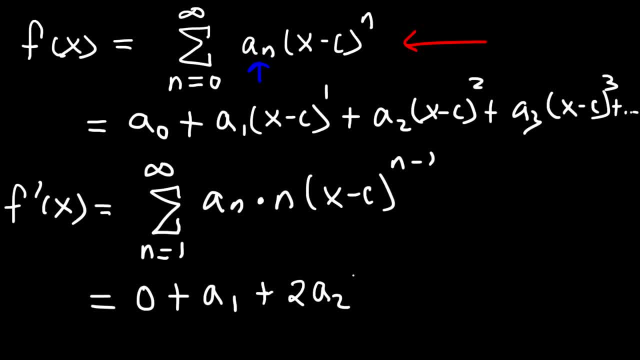 So we're going to have 2 times a2 x minus c to the first power, And then the derivative of this term is going to be 3 times a sub 3 x minus c to the second power, And this will continue. Now you might be wondering: why are these n values different? 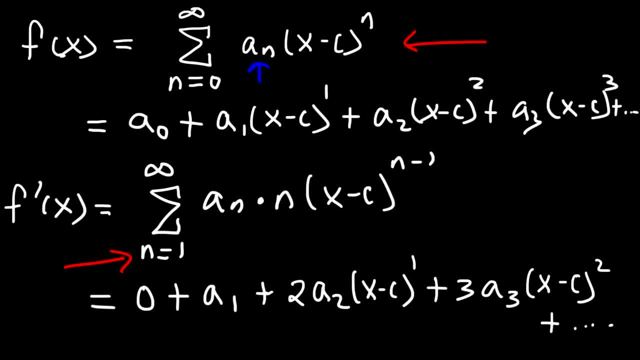 We started with n equals 0, but now we have n equals 1.. Why is that? Well, if we plug in 0 into this expression for n, what will we get? a sub n times 0 times. whatever this is, all of that is going to be 0. 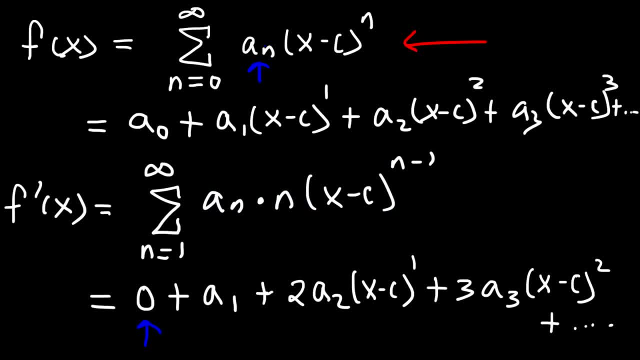 And so that's going to give us the first term, which is the derivative of a sub 0.. Now, 0 plus a sub 1 is still going to be a sub 1.. So we can just, Let's just get rid of this. 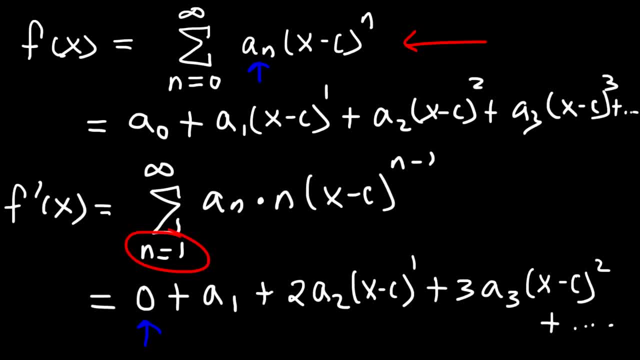 So if you start with n equals 0, it's not going to change your answer. You can still get the right answer. But it's just. We can neglect it. It's not important, Because the real value starts when n equals 1.. 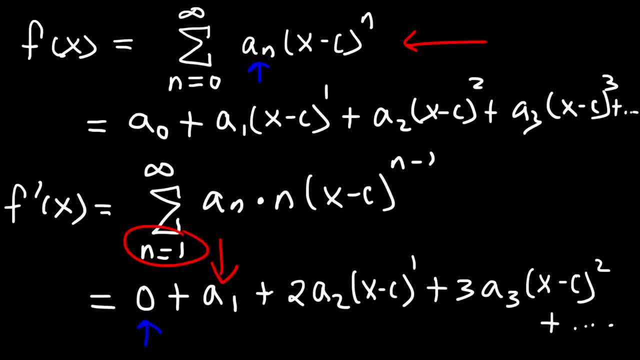 So you can put n equals 0 or n equals 1.. It's up to you. Now let's talk about integrating a power series. So let's find the antiderivative of f1.. f of x, dx. So what is the antiderivative of that general expression? 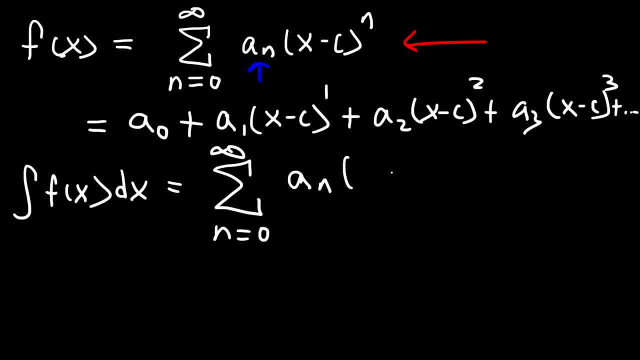 Well, we can rewrite the constant And then we just got to use the power rule for integration. So we need to add 1 to n, So it's going to be n plus 1, and then divide by that result. Now, just like I mentioned before, you can list out the terms based on this expression. 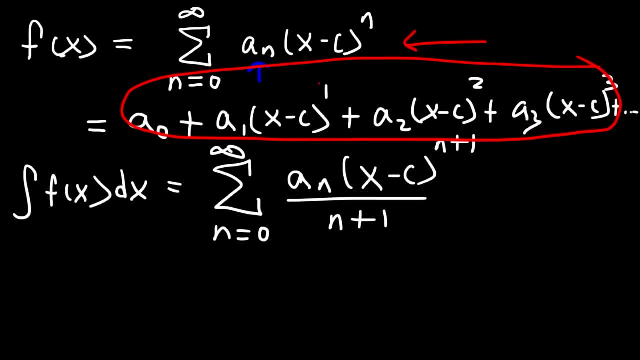 Or you can find the antiderivative of f1.. Or you can find the antiderivative of each term in the series. So let's do it that way. So what is the antiderivative of a sub 0?? Now you might be thinking it's a sub 0 times x. 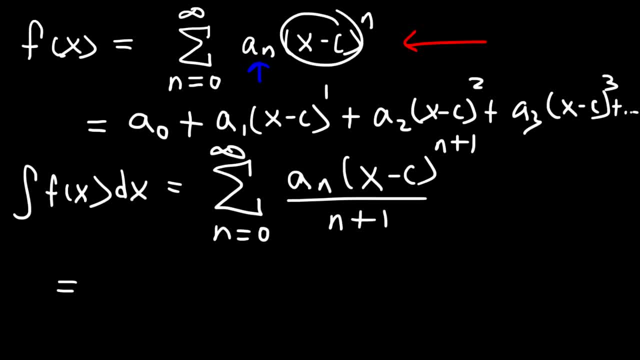 Which is true, But for this series it's centered at c, So it's going to be a sub 0 times x minus c. By the way, there's one thing that I almost forgot to write, And that is whenever you're looking for an indefinite integral. 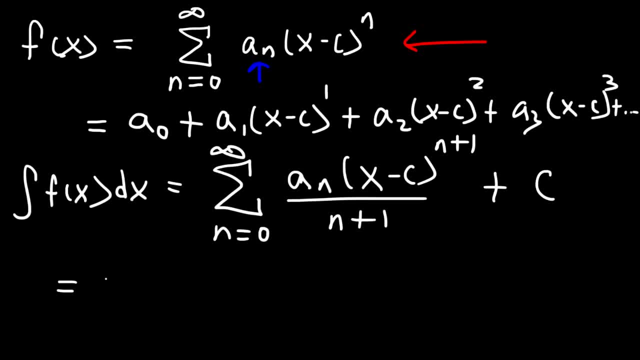 you need to add the constant. So this is the constant of integration. So let's put that first. So we're going to have a sub 0 times x minus c to the first power. Now what about the antiderivative of that expression? 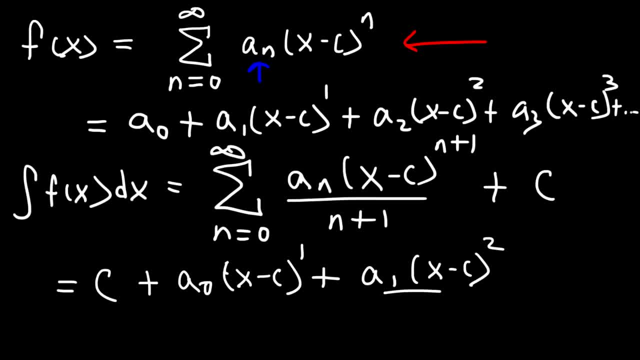 It's going to be a sub 1 times x minus c to the second power over 2.. And then, for this one, it's going to be a sub 2 x minus c to the third power over 3.. And then, for the last one, it's going to be a sub 3 x minus c to the 4th power over 4.. 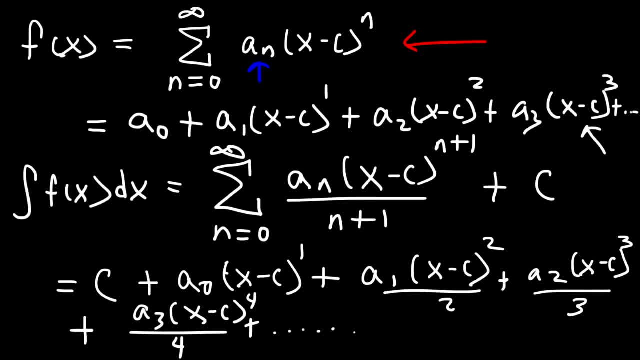 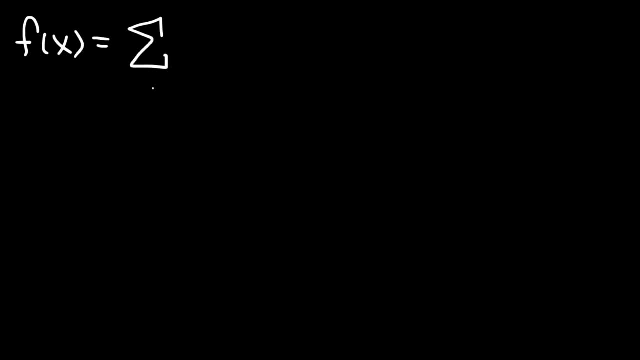 And then this will go on forever, so the pattern will just continue to repeat. And so that's how you can integrate a power series. You could just simply use the power rule for integration. Let's say that f of x is the power series from 1 to infinity, x to the n over n, factorial. 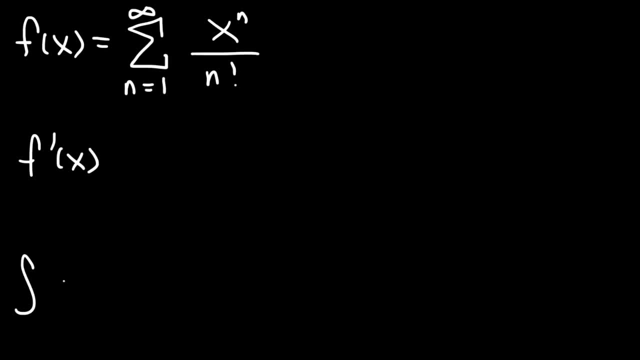 What is f prime of x And what is the integral of f of x- dx, represented as a power series? Now you need to know that n is a constant but x is the integral of f of x dx. So you need to find the derivative of x to the n. 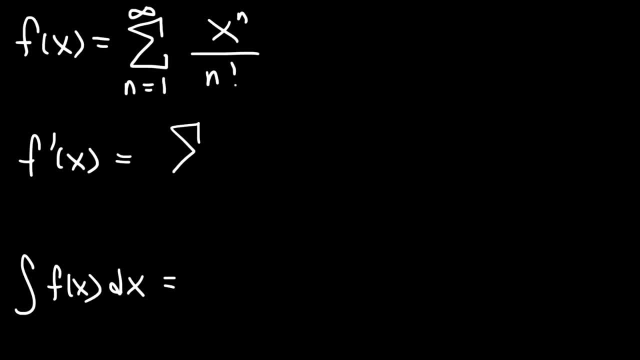 The derivative of x to the n. well, first let's rewrite the sigma notation and the summation symbol. The derivative of x to the n is going to be n times x to the n minus 1.. Now n- factorial. we said it's a constant, so we're just going to rewrite it in the bottom. 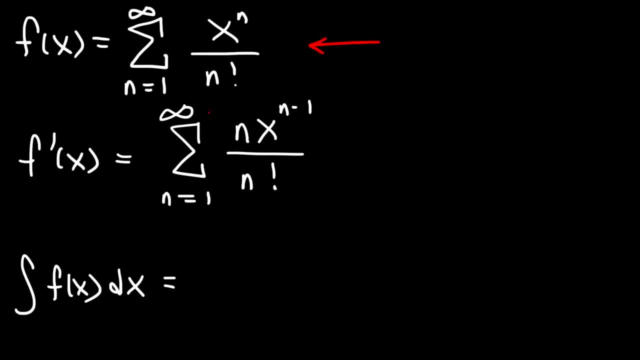 Now what about the integral of this power series? So let's focus on finding the antiderivative of x to the n, So that's going to be x to the n plus 1 divided by n plus 1.. And then rewrite this on the bottom. 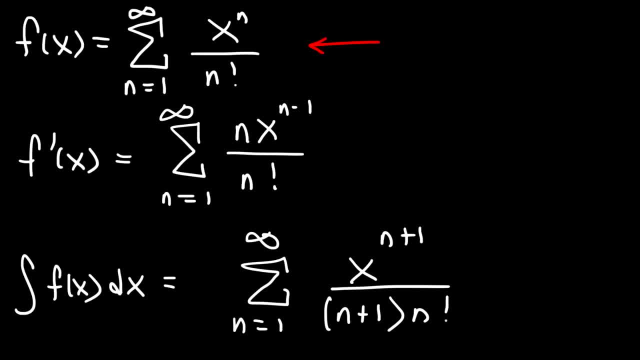 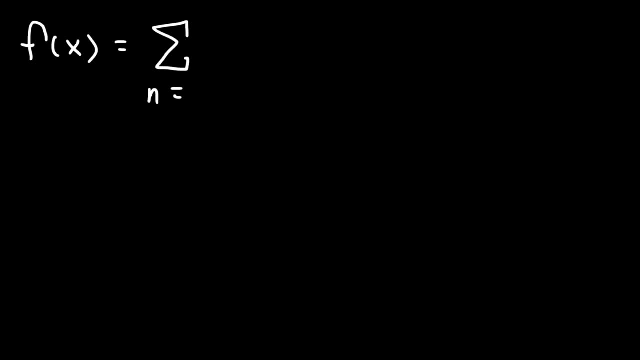 So we're going to say times n, factorial, And so that's how you can find the derivative and the integral of that expression. Let's work on what we're going to do next. One more problem, just like the last one. So let's say that f of x is represented by the power series. 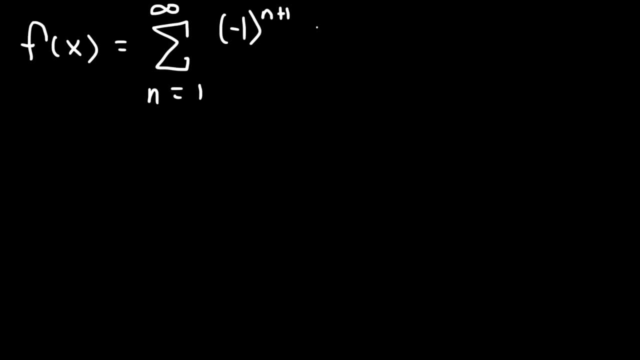 negative 1 to the n plus 1 times x raised to the 2n, divided by 5 to the n. So let's start with f. prime of x. So what's the derivative of that expression? So, using the power rule, we're going to rewrite the constant. 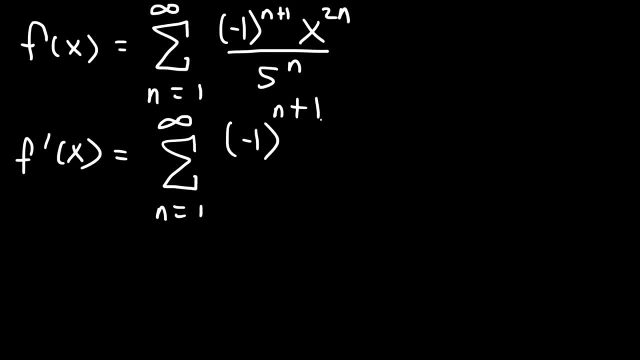 negative: 1 to the n plus 1, that's a constant. There's no x variable associated with it, And 5 to the n is a constant. Now, x is the variable. So what is the derivative of x to the 2n? 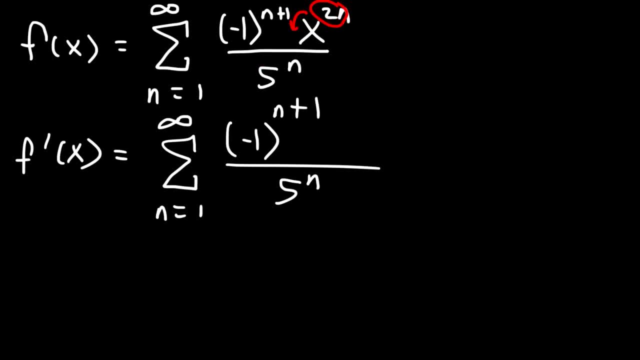 Well, we're going to have to take the exponent 2n, move it to the front, And so it's going to be times 2n, and then x to the 2n minus 1.. And so that's the derivative of this expression. 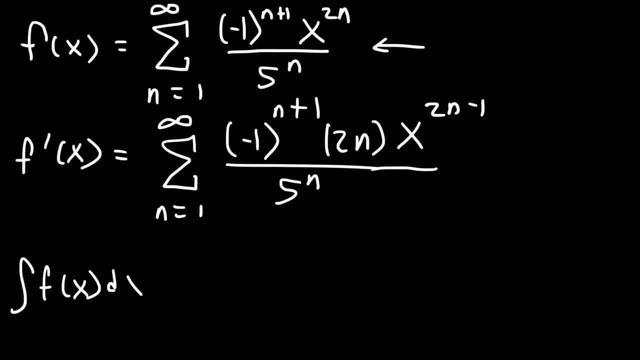 So now let's find the integral of f, of x, dx. So let's rewrite all the constants Negative, 1 to the n plus 1 times, I mean divided by 5 to the n, And then the antiderivative of x to the 2n is going to be x to the 2n plus 1. 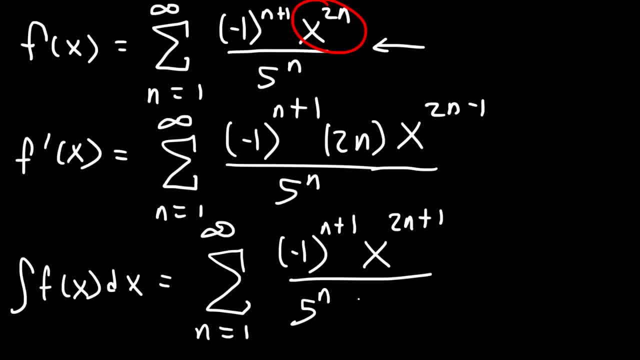 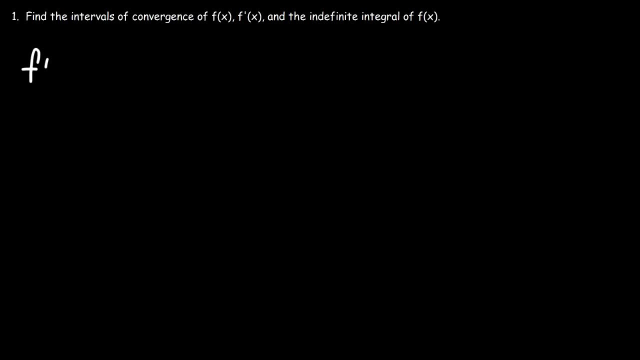 and then divided by that result, or divided by 2n plus 1.. And so this is the integral for f of x, dx. Now let's work on some practice problems. Let's say that f of x is the power series from 1 to infinity. 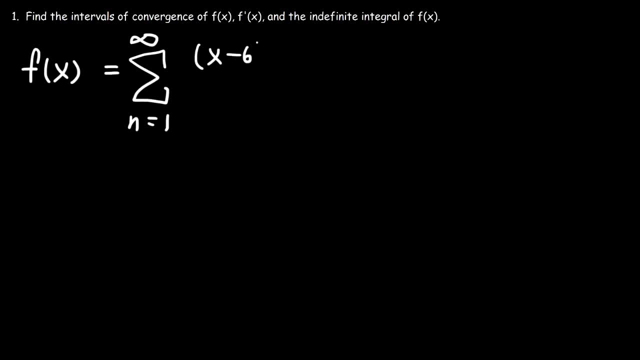 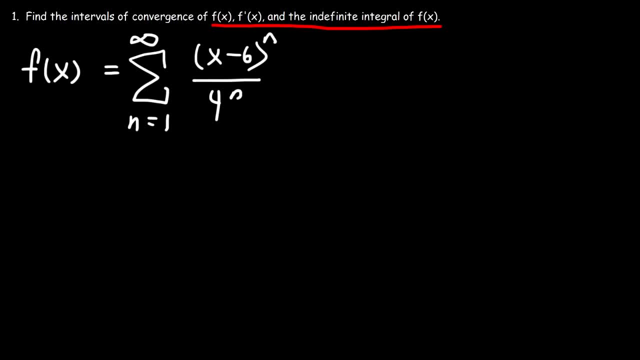 Convergence, Convergence, Convergence, Convergence, Convergence. f, prime of x and the integral of f of x. So let's start with the original function f of x. How can we determine the interval of convergence? The first thing: 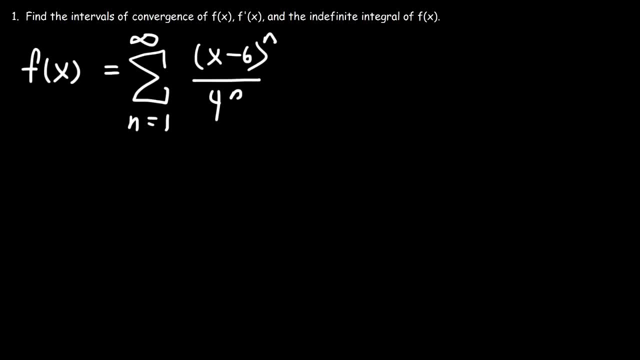 we need to use is the ratio test. We need to show where the ratio test is less than 1, because that's where the series is going to converge. So, if you recall, it's going to be the limit, as n goes to infinity, of u sub n plus 1 divided by u. 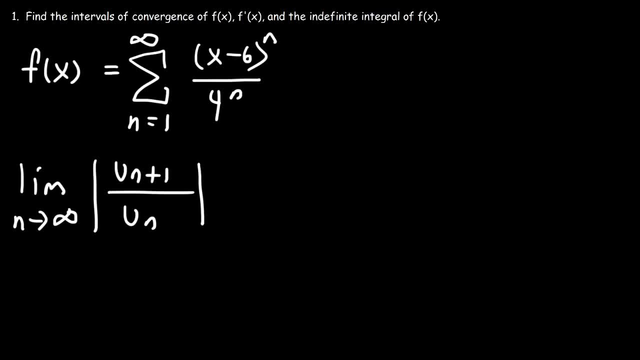 sub n. Now u sub n plus 1 is basically this expression, but all we need to do is replace n with n plus 1.. So we're going to have the limit as n goes to infinity, and then it's going to be x minus 6 to the n plus 1 over 4 to the n plus 1.. So 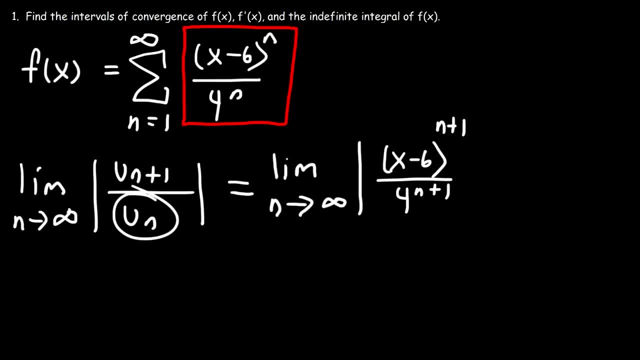 that's u sub n plus 1, and then we need to divide it by the original equation. So how can we simplify this expression? What do we need to do? x minus 6 raised to the n plus 1.. We can rewrite that as x minus 6 to the n times x minus 6 raised to the first power And 4 to the n plus 1.. Let's write that as 4 to the n plus 1.. 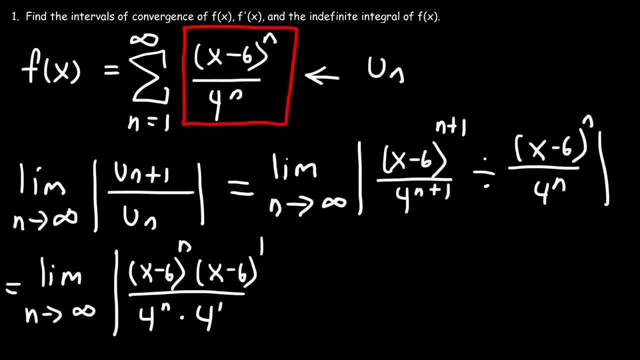 to the n times 4 to the first power. And then we need to change division to multiplication and then flip the second fraction. So now we can cancel x minus 6 to the n power and also 4 to the n. Now we have left over is the limit plus 4 to the n. 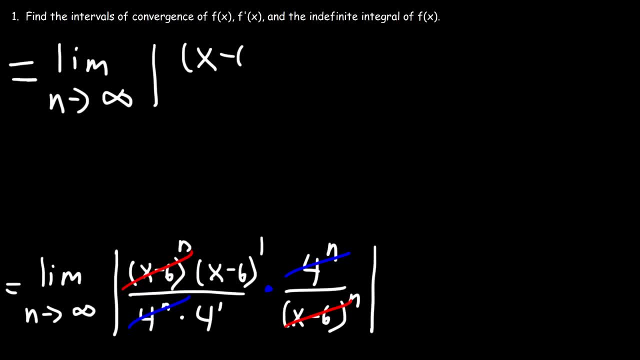 as n goes to infinity, of x minus 6 divided by 4, all within the absolute value expression. Now notice that n is not part of this expression, so we don't need the limit expression anymore. As n goes to infinity, this is still going to be the absolute value of x minus 6 over 4.. 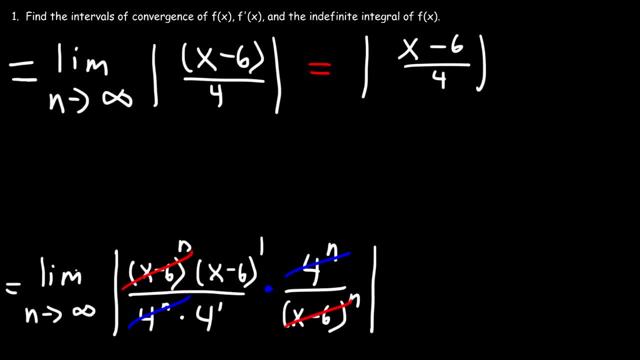 Now we could take the constant 4 and just move it to the outside. So what we now have is 1 fourth times the absolute value of x minus 6.. Now we want to know when this expression converges, And so, according to the ratio test, the series will converge if the limit is less than 1.. 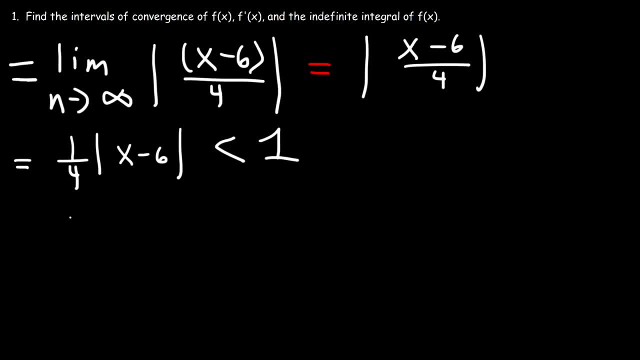 So now we need to solve for x. Let's multiply both sides by 4.. Just to get rid of the 1 fourth on the left. So we have the absolute value of x minus 6 is less than 4.. Notice that it's in the form: x minus c is less than r. 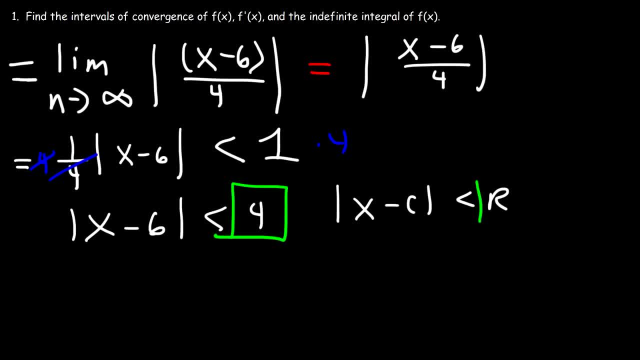 So the radius of convergence is 4.. Now at this point we can write that expression as: x minus 6 is less than 4, but also greater than negative 4.. So now we need to add 6 to both sides. 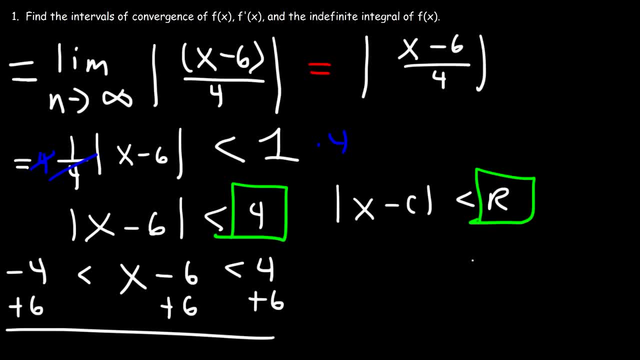 Or rather all 3. All 3 sides. And so x is less than 4 plus 6,, which is 10,, but greater than negative 4 plus 6,, which is 2.. So right now we have this particular interval of convergence. 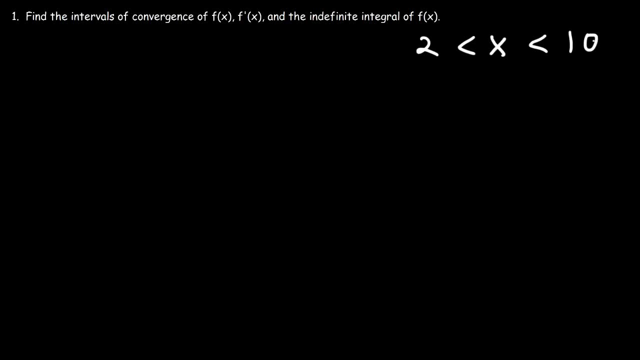 So x is between 2 and 10. And the radius of convergence is 4. And it's centered at 6. Because of the x minus 6 expression. So let's rewrite the original series. So just by looking at this part you can tell that it's centered at 6.. 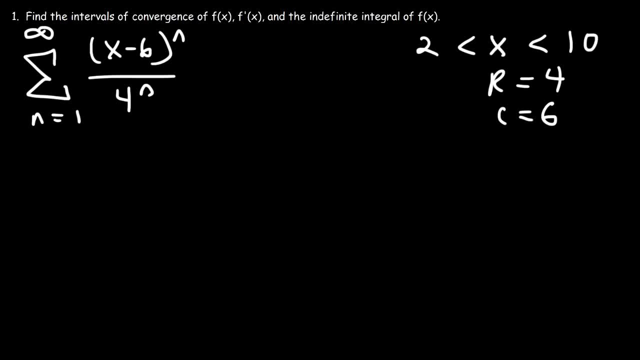 Now, in order to determine the interval of convergence, we need to check the endpoints 2 and 10.. So let's plug in 2 and see if the power series converges when x is equal to 2.. So this is going to be 2 minus 6, raised to the n, over 4 to the n. 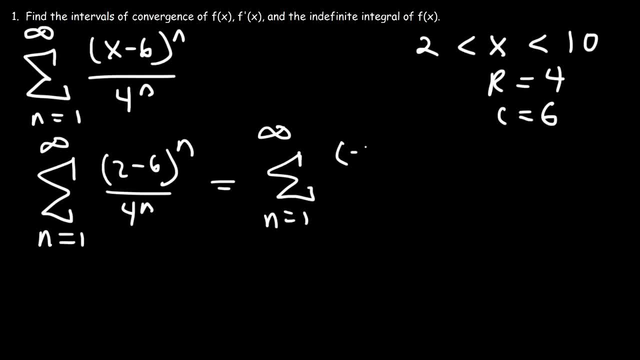 2 minus 6 is negative 4.. So we have negative 4 to the n over 4 to the n, And so we can write that as negative 4 over 4 to the n. And so this simplifies to negative 1 to the n. 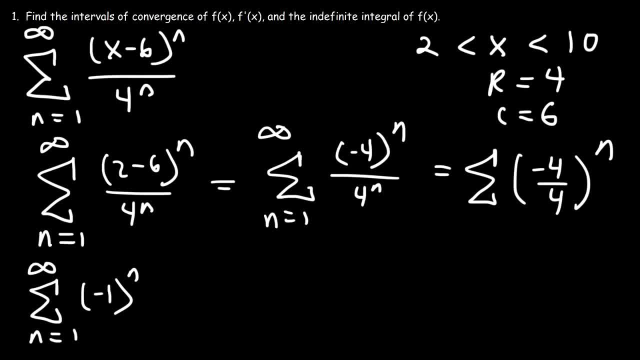 Now, what type of series do we have? Notice that this is in the form of a geometric series. So this is a times r raised to the n minus 1.. So you can see that r is negative 1.. Now, what do we know about the convergence of a geometric series? 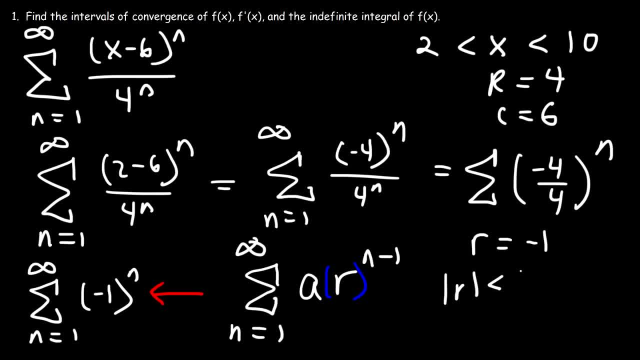 If the absolute value of r is less than 1, then the series will converge. Now, if the absolute value of r, the common ratio, if it's greater than or equal to 1, the series will diverge. So the absolute value of negative 1 is equal to 1.. 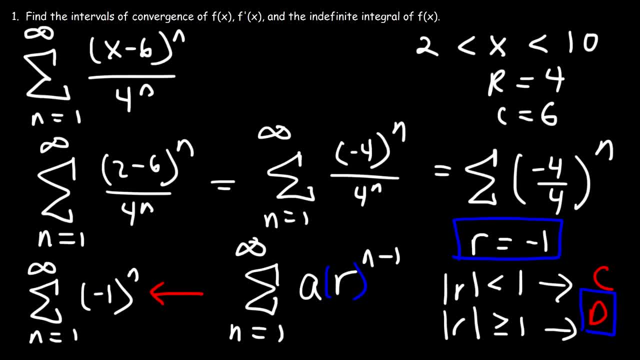 So therefore, we can say that this particular series diverges. So when x is 2, the geometric power series diverges. So when x is 2, the geometric power series diverges. But when x is greater than 2, then you're going to get something. the common ratio will be less than 1.. 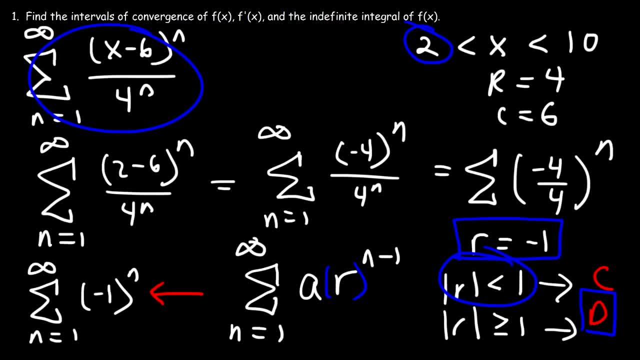 And so it's going to converge. That is, the absolute value of this- will be less than 1.. For example, let's say, if we pick a number between 2 and 10.. Let's say 5.. If I were to plug in 5, 5 minus 6 to the n over 4 to the n, that's going to be negative: 1 to the n over 4 to the n. 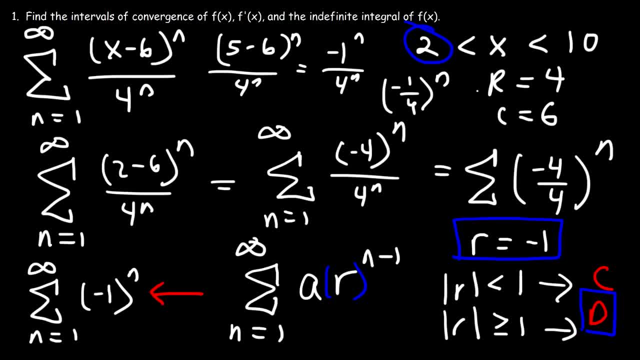 Which is negative 1 to the n over 4 to the n. So my common ratio is negative 1 fourth, which means the absolute value of that is 1 fourth and that's less than 1.. So when x is 5, the geometric power series converges. 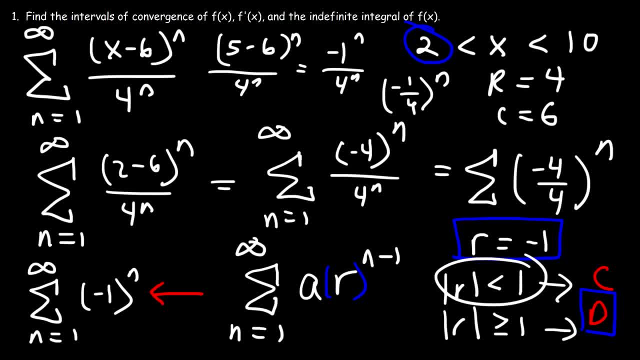 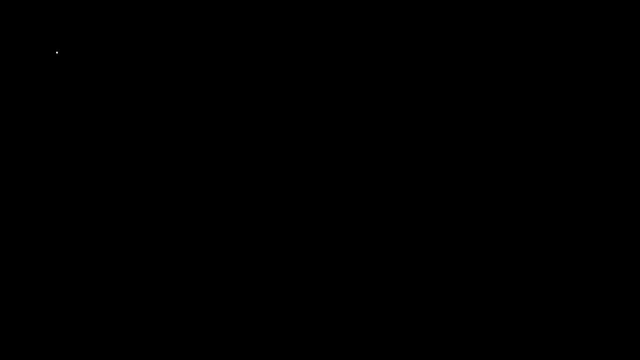 So when x is between 2 and 10, it's going to converge, But when x is equal to 2,, as we see here, it diverges. Now let's check the other endpoint. When x is equal to 10, will it converge or diverge? 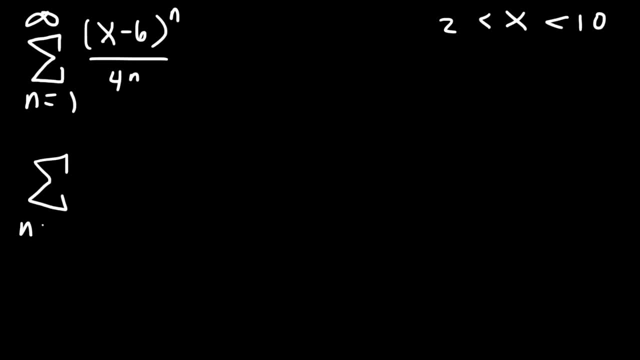 So let's replace x with 10.. So this is going to be 10 minus 6 to the n over 4 to the n. Now 10 minus 6 is 4.. So we have 4 to the n over 4 to the n, which we can rewrite that as 4 over 4 to the n. 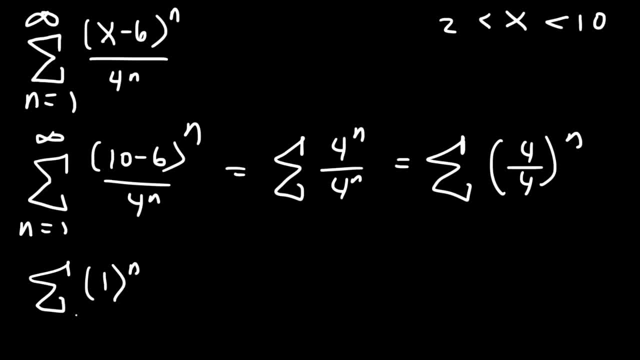 And so we're going to have 1 to the n. So in this case, for the geometric series, the common ratio is 1.. And so, since the absolute value of r is equal to or greater than 1,, it still diverges. 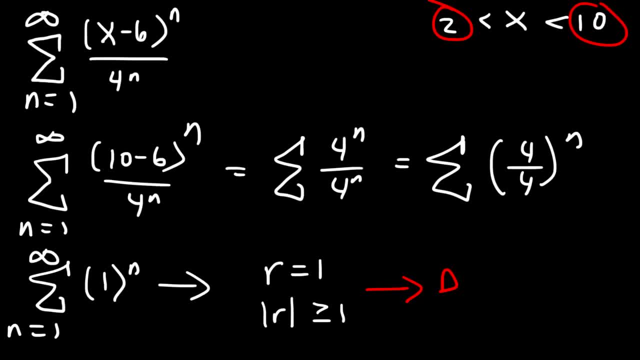 So 2 and 10 are not included, because when x is equal to 2 or when x is equal to 10, the geometric power series diverges. So therefore the interval, So therefore the interval, The interval of convergence, is 2 to 10.. 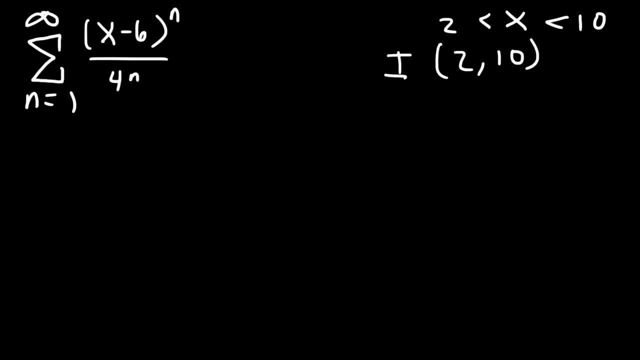 Now, if you want to graph it, let's say, on a number line, it's going to look like this: So the geometric power series is convergent from 2 to 10, but centered at 6.. So this is our x equals c value. 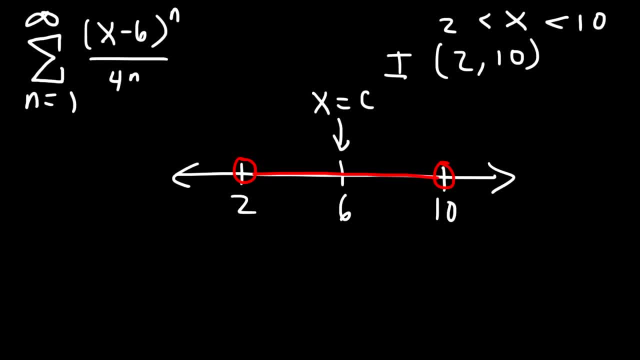 And we're going to have an open circle at 2 and 10.. And the radius, The radius of convergence, is 4.. So that's it for f of x. Now let's find the interval of convergence for the derivative of f or f, prime of x. 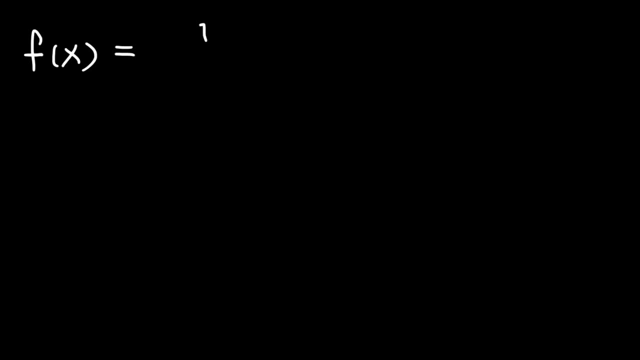 So we said that f of x is represented by the power series from 1 to infinity of x minus 6 raised to the n, divided by 4 raised to the n. Okay, So in this case, what is the derivative of that expression? 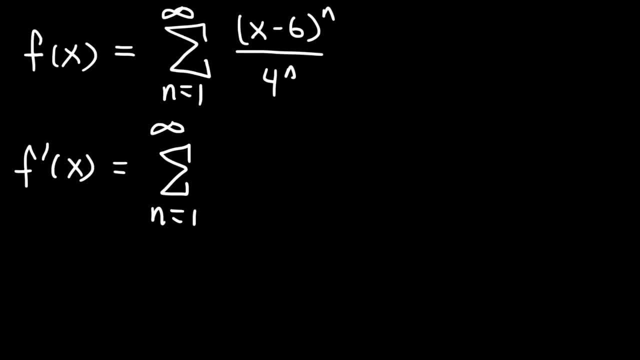 So what is the derivative of x minus 6 raised to the n, over 4 to the n? So first you need to realize that n is a constant but x is a variable. So we're really differentiating x minus 6 to the n power. 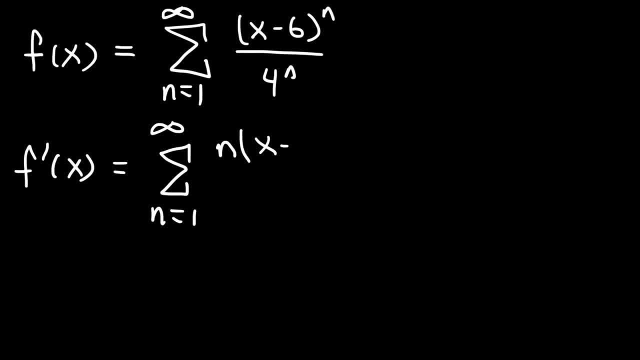 So, using the power rule, it's going to be n? x minus 6 to the n minus 1 power And the constant 4 to the n. we're just going to rewrite. Now let's determine the interval of convergence for this expression. 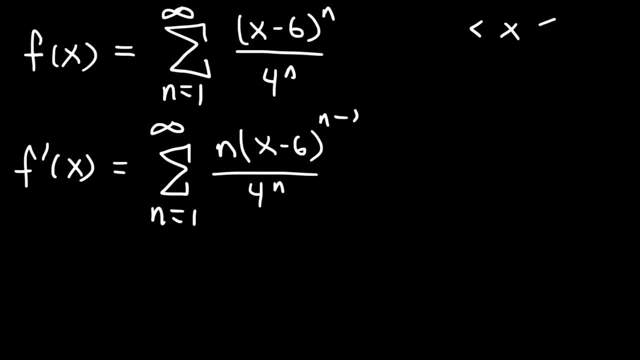 It turns out that it's going to be very similar to the interval of convergence for the original expression, But let's use the ratio test to confirm it. So let's take the limit, as n goes to infinity, of u sub n plus 1.. 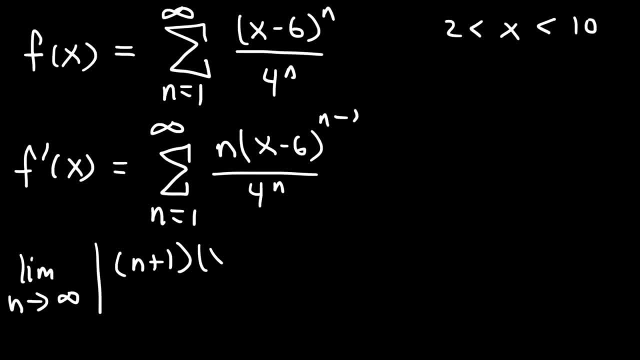 So that's going to be n plus 1 times x minus 6.. And then, And this is going to be n plus 1 minus 1.. So I'm just going to write it just like that, Divided by 4 to the n plus 1.. 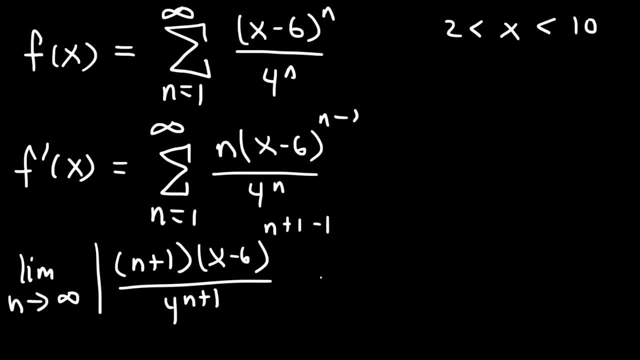 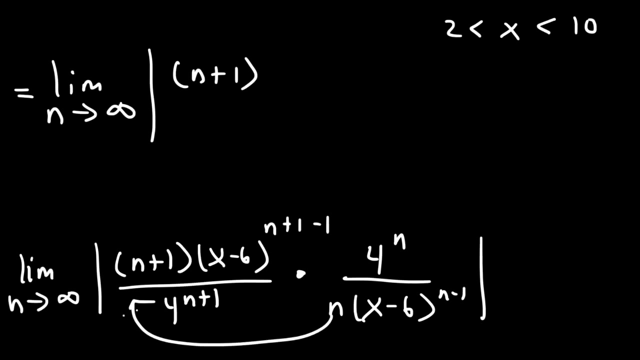 And then it's divided by u sub n or multiplied by the reciprocal of u sub n, which is 4 to the n times this expression. So how can we simplify this particular limit? So we have n plus 1.. And I'm going to put the n under that. 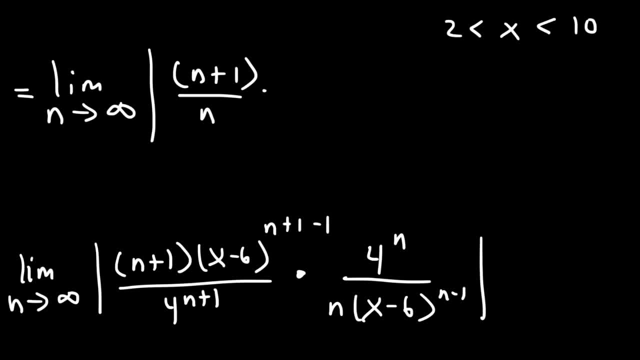 So n plus 1 over n And then x minus 6 raised to the n plus 1 minus 1.. I'm going to write that as x minus 6 to the n plus 1.. I mean not n plus 1, but n minus 1 times x minus 6 to the 1 power. 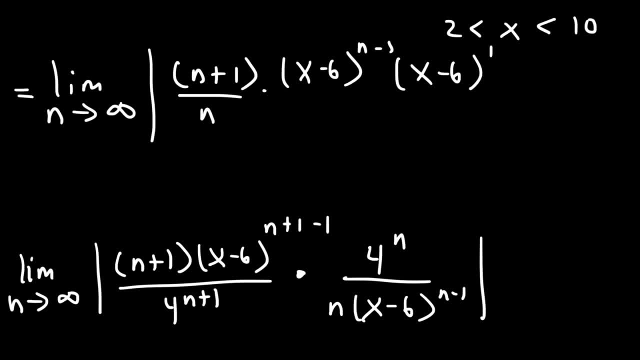 Now, the reason why I wanted to write it that way is so that it matches with what we see there. Now I also have 4 to the n on the numerator of the second fraction. On the bottom I have 4 to the n plus 1,. 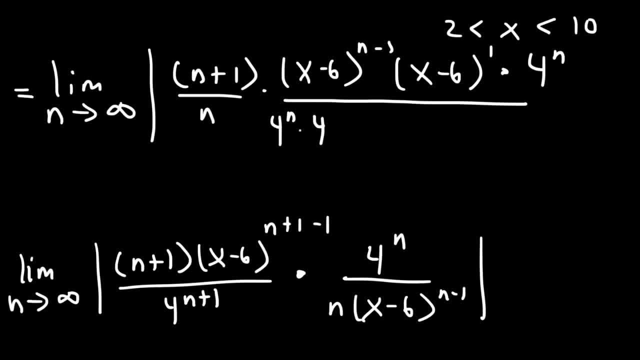 which I'm going to write that as 4 to the n times 4 to the first power. And then I also have this expression: And x minus 6 raised to the n plus, I mean n minus 1.. So I can cancel x minus 6 raised to the n minus 1.. 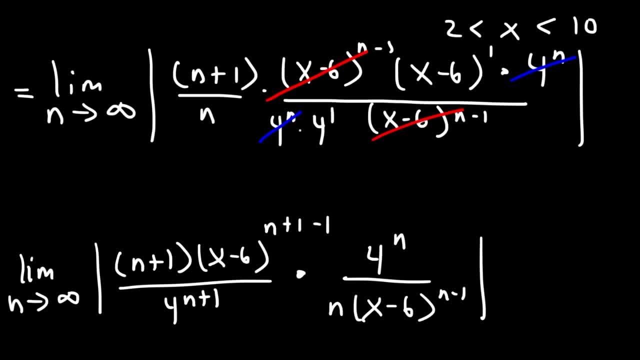 And also 4 raised to the n. At this point I'm going to separate it into two separate absolute value expressions, So this is going to be one of them. So we have the absolute value of n Plus 1 over n. 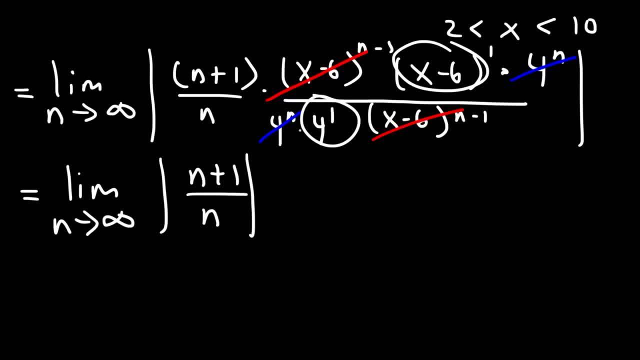 And then for the other expression, x minus 6 over 4.. Now, as n goes to infinity, what happens to n plus 1 divided by n? That goes to 1.. This one is insignificant when n becomes very large, And so you're going to get n over n, which is 1.. 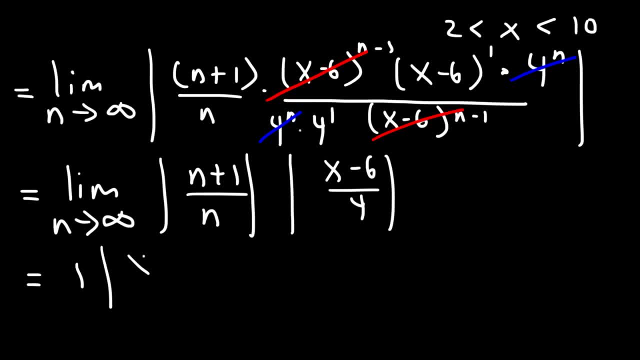 So what we now have is 1 times the absolute value of x minus 6 over 4.. Which we can write that as 1 fourth absolute value, x minus 6.. And because we're dealing with the ratio test and we want to find the x values where the series will converge, 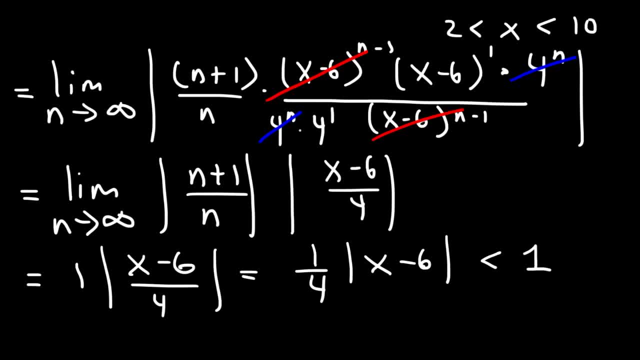 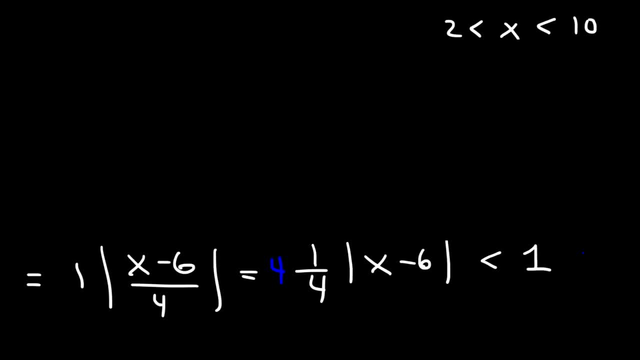 we need to set it less than 1.. So if we multiply both sides by 4, we're going to get the same result. So 4 times 1, fourth, that's 1.. And so we have: the absolute value of x minus 6 is less than 4.. 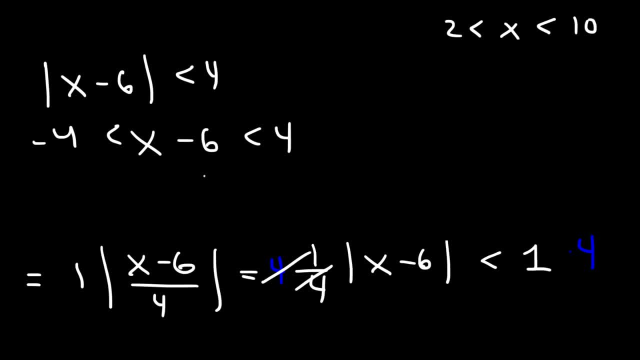 Which means x minus 6 is between 4 and negative 4.. Add in 6 to all three sides: 4 plus 6 is 10.. Negative 4 plus 6 is 2.. And so, as you can see, the interval of convergence is the same for f of x. 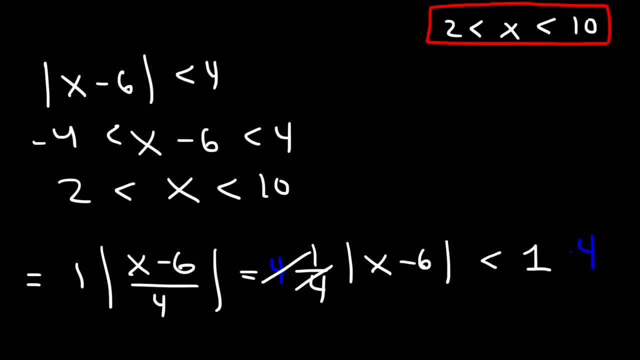 And f, prime of x. The only thing that may be different are the endpoints, So let's write the original series for the first derivative, Which we found it to be this. So here's the question for you: When x is 2, will the series converge? 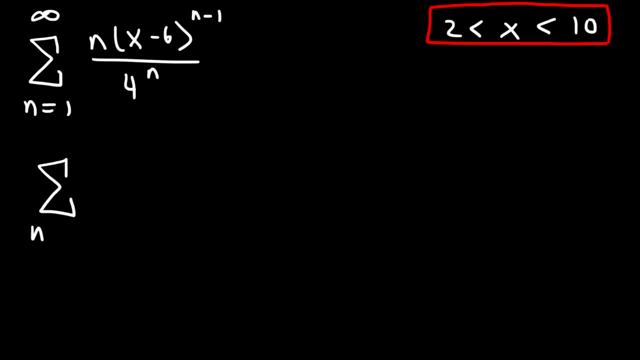 Or will it diverge? So this is going to be: n. 2 minus 6 is negative 4 to the n minus 1 over 4 to the n. So we have negative 4 to the n minus 1.. 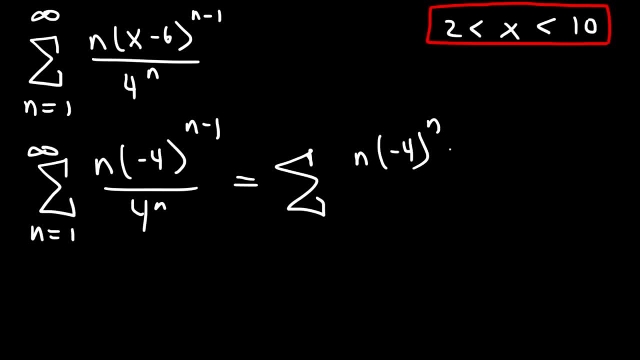 We can write that as negative 4 to the n times negative 4 to the negative. 1 power over 4 to the n. So we can write negative 4 to the n over 4 to the n as negative 4 over 4 raised to the n. 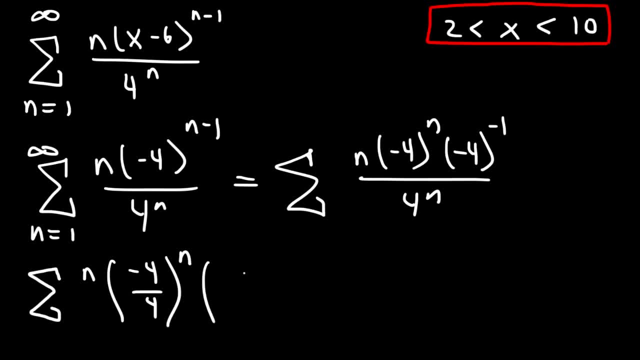 And negative 4 to the negative 1 power. that's basically 1 over negative 4 to the first power. So by moving negative 4 to the bottom, the negative exponent becomes positive. Negative 4 divided by 4, that's negative 1.. 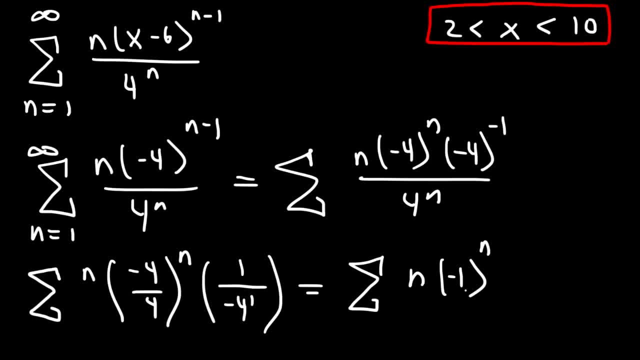 So this is going to be negative 4 to the n minus 1 over 4 to the n. So we have negative 1 to the n and then times or just divided by negative 4.. Now I'm going to rewrite it like this: 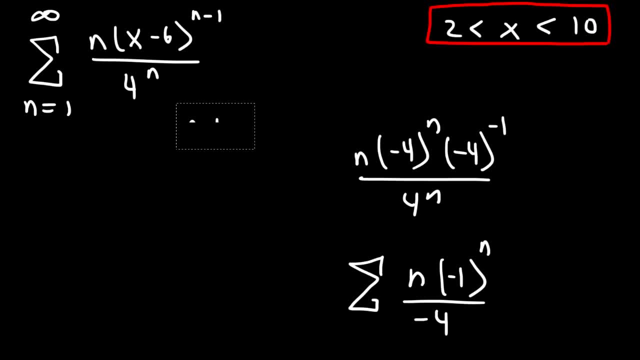 Negative 4 is basically 4 times negative 1.. So now we have n times negative 1 to the n times negative 1, which is negative 1 to the first power over 4.. So this is negative 1 to the n plus 1 times n divided by 4.. 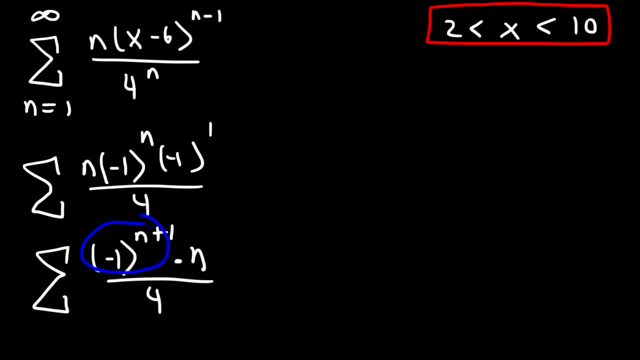 So notice the negative 1 to the n plus 1.. That tells us that we're going to have alternating signs in the series. So we have an alternating series, which means we need to use the alternating series test to see if it's going to converge or diverge. 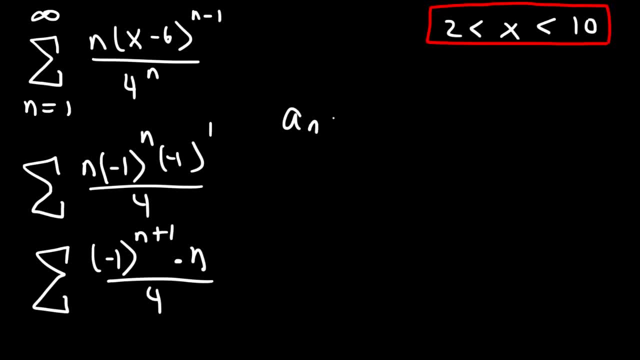 Now for the alternating series. our a sub n is everything except this portion which alternates the sign. So our a sub n is n over 4.. The first thing we need to do is make sure that it passes the divergence test. 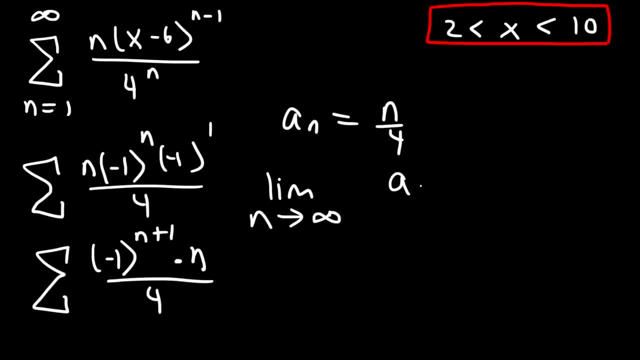 So the limit as n approaches infinity, For a sub n, it has to equal 0. So let's see if it does As n goes to infinity. what happens to n divided by 4? Infinity divided by 4 is still infinity. 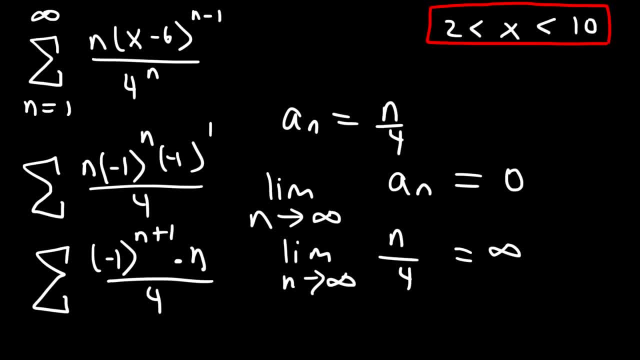 So therefore it does not pass the divergence test And as a result, it will now pass the alternating series test. So this series Diverges when x is equal to 2.. So 2 is not included in the interval of convergence. 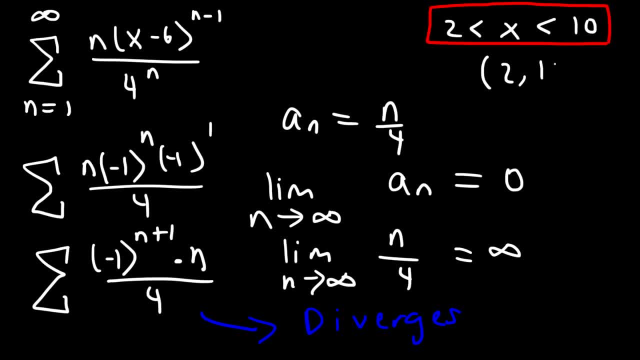 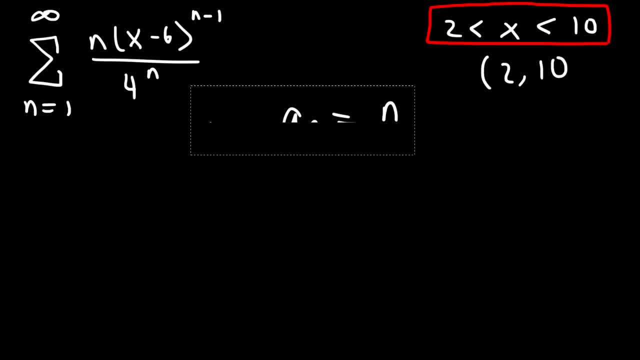 So we're going to use a 2 in parentheses as opposed to a bracket. So now, what about when x is equal to 10? Let's see what's going to happen. So we're going to have n, and then 10 minus 6 is positive 4.. 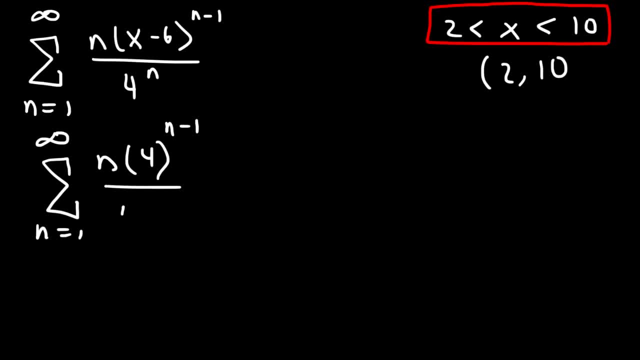 So positive 4.. So 4 to the n minus 1 over 4 to the n, So 4 to the n minus 1 over 4 to the n. we need to subtract the two exponents: n minus 1 minus n is just going to be minus 1.. 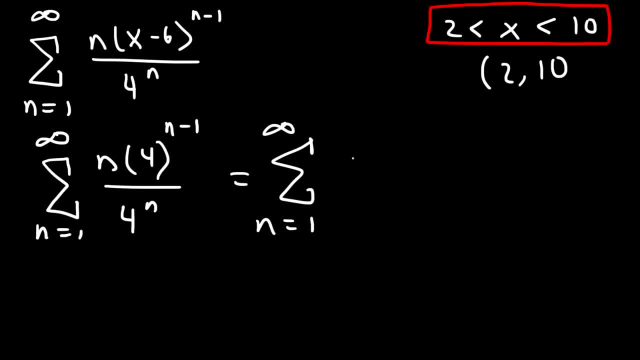 The 4 to the n's will cancel, And so we're going to get n times 4 to the negative 1 power, or simply n over 4.. So what test Should we use to see if the series will converge or diverge? 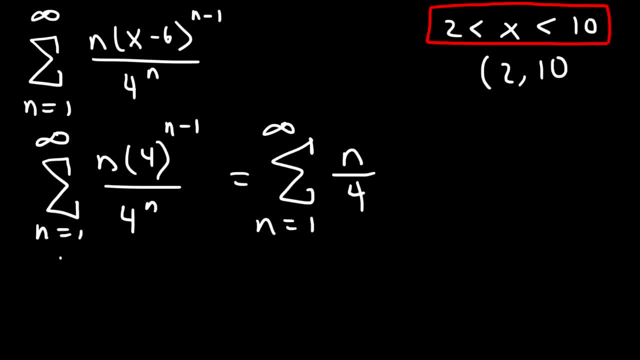 The most easiest one to use is the divergence test. If we take the limit as n goes to infinity for n over 4, we know it's going to be infinity, And so the series diverges. So it diverges at 2 and 10, but it converges between 2 and 10.. 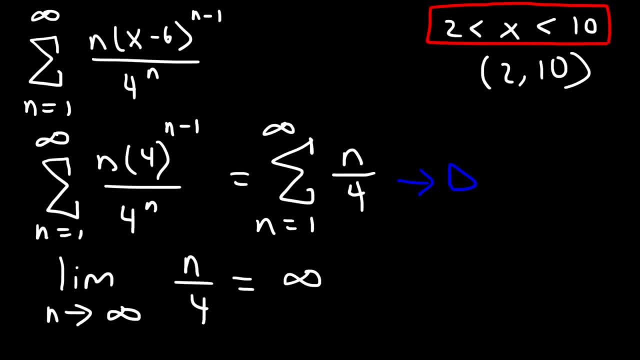 So f, prime of x and f of x, for this particular example, have the same interval. Keep in mind, though, the endpoints may vary. Sometimes they're the same, sometimes they're different. So now let's move on to the integral of f of x. 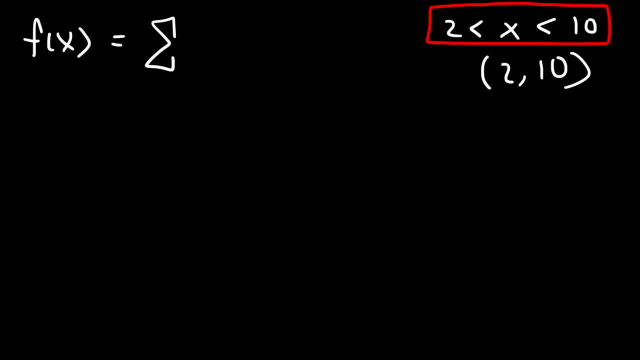 So let's start with the original power series And then let's find the integral of f, of x, dx. So we need to use the power rule. So we're going to add 1 to n, So this is going to be n plus 1.. 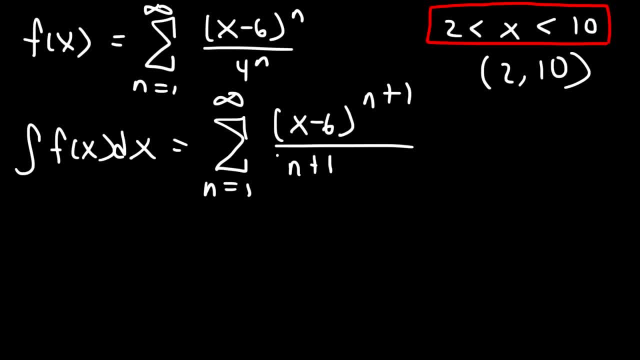 And then we're going to divide by n plus 1.. Now 4 to the n is a constant, so we're just going to rewrite it exactly where it was. So this is our new series. Now, if you perform the ratio test on this series, following the same steps that we employed, 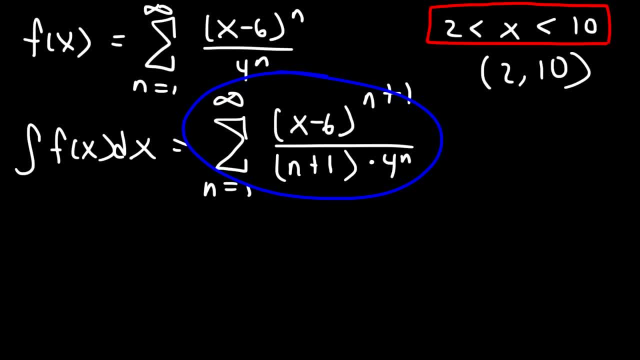 for f of x and f prime of x, you're going to get the same inequality from 2 to 10.. The only thing we need to do now is we need to check the endpoints 2 and 10.. So let's go ahead and plug in 2 into the power series. 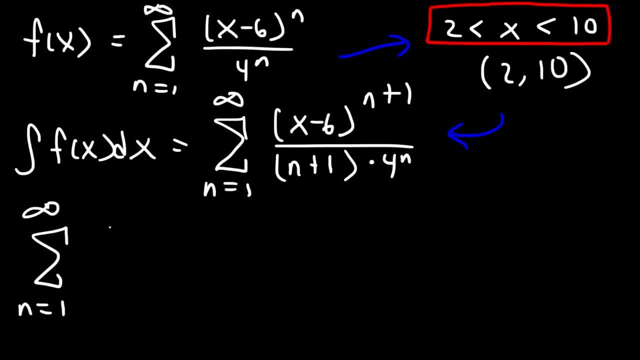 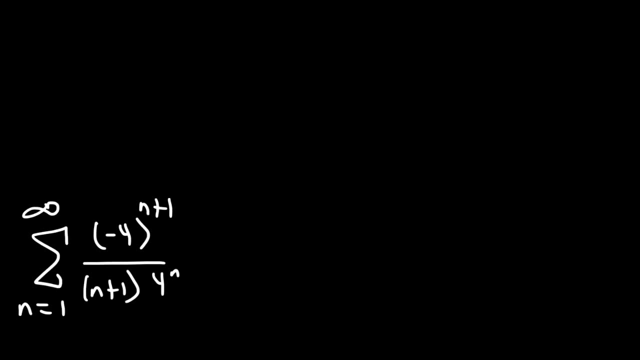 So this is going to be 2 minus 6, which is negative 4, to the n plus 1, over n plus 1.. n plus 1 times 4 to the n. So what does that simplify to? 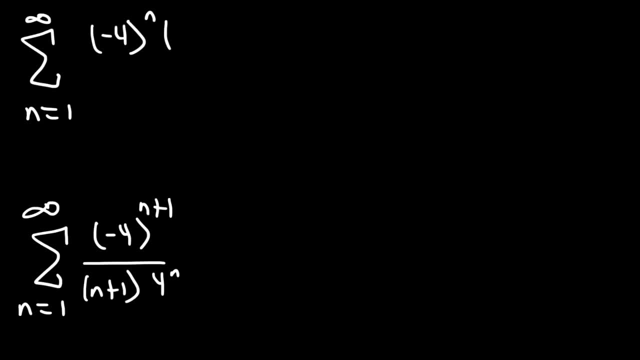 So this is going to be negative 4 to the n times negative 4 to the first power over n, plus 1 times 4 to the n. So if we divide these two negative 4 divided by 4 is negative 1.. 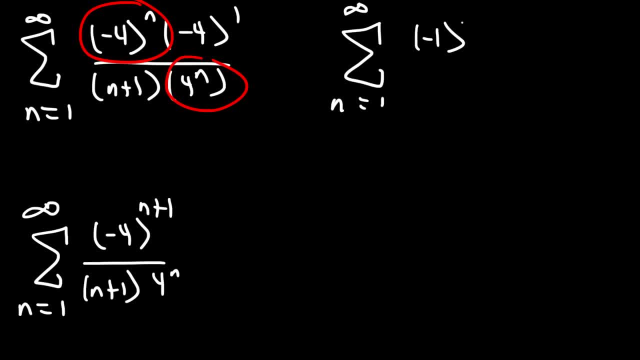 And so that's going to be negative 1 to the n power. And then we have negative 4 over n plus 1.. Negative 4, I'm going to write that as 4 times negative 1 to the first power. 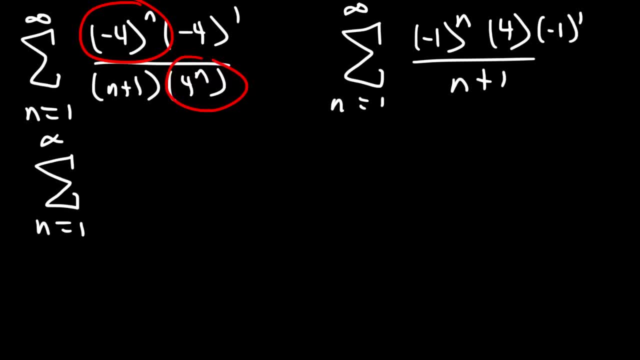 So we can write this series like this. So we can write this series like this. This is going to be negative 1 to the n plus 1 times 4 over n plus 1.. So will the series converge or will it diverge? 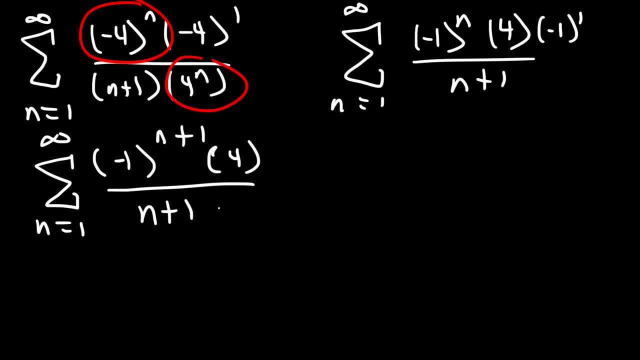 What would you say? Negative 1 to the n plus 1, that tells us that we have an alternating series. So will it converge or will it diverge? So let's perform the divergence test. So if we take the limit as n goes to infinity for a sub n, which is everything except this part, so that's 4 over n plus 1, what's going to happen? 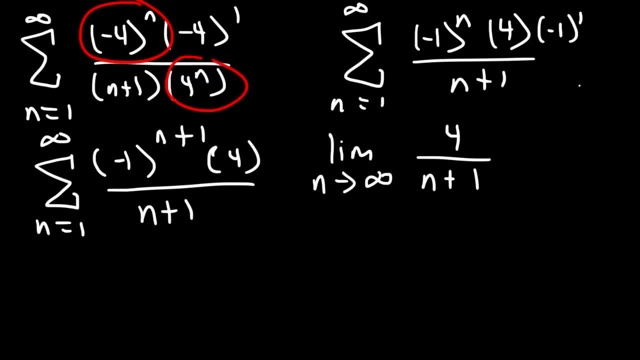 When n becomes very large, 4 over n plus 1, that's going to go to 0. So it passes the first part of the alternating series test. Now for the second part. we need to show that a sub n is a decrease in sequence. 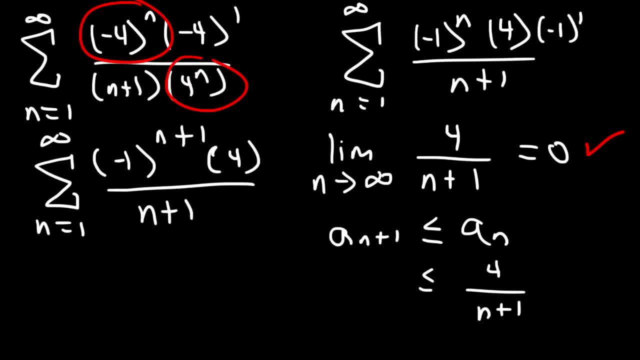 So a sub n is 4 over n plus 1.. And the next term a sub n plus 1, that's going to be 4 over n plus 2.. 4 over n plus 2 is always less than 4 over n plus 1.. 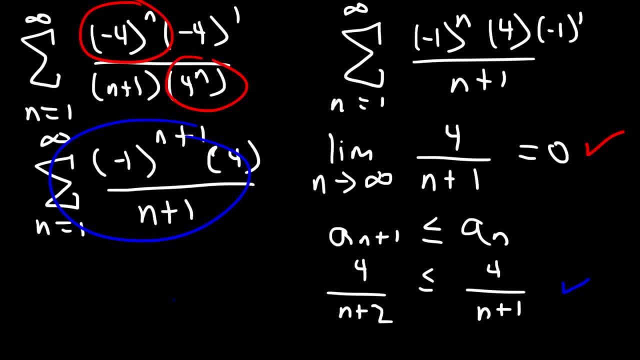 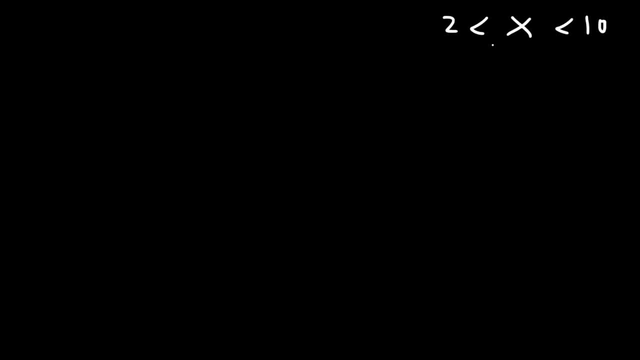 So by the alternating series test this series converges. So therefore 2 is included in the interval of convergence for the integral of f of x, dx. So it's a little different than the last two. Now let's rewrite our power series. 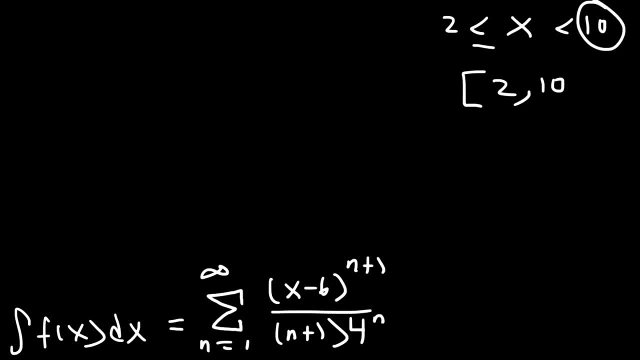 So what about if f of x is 10.. Will the power series converge or will it diverge? So let's plug in 10.. 10 minus 6 is 4.. So we're going to have 4 to the n plus 1, which I'm going to write that as 4 to the n times 4 to the first power over n, plus 1 times 4 to the n.